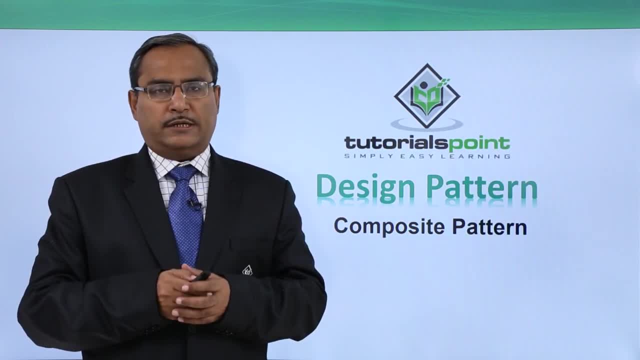 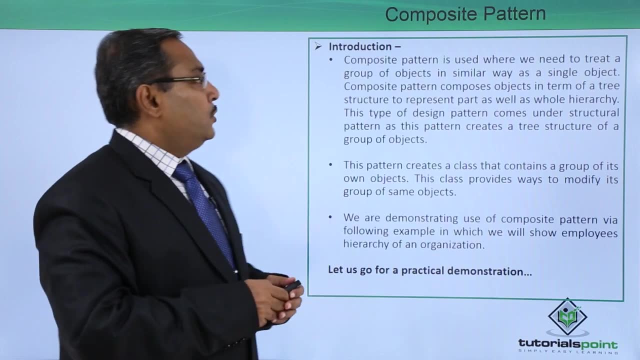 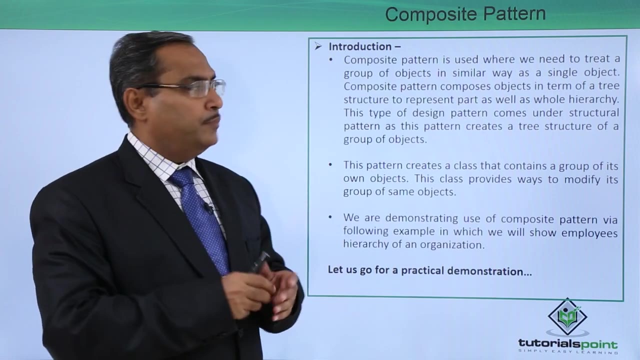 Composite design pattern. In case of composite design pattern, we shall treat a group of objects in a similar way as a single object. Composite pattern is used where we need to treat a group of objects in a similar way as a single object. Composite pattern composes objects in terms of a. 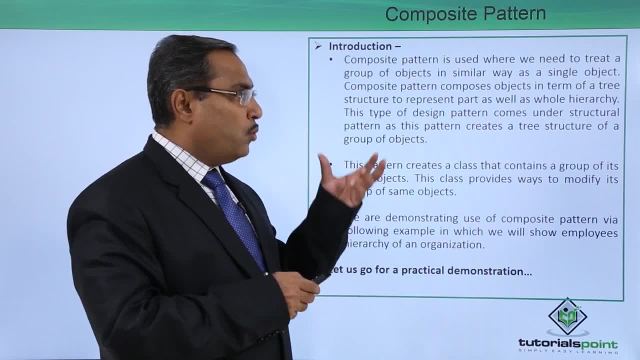 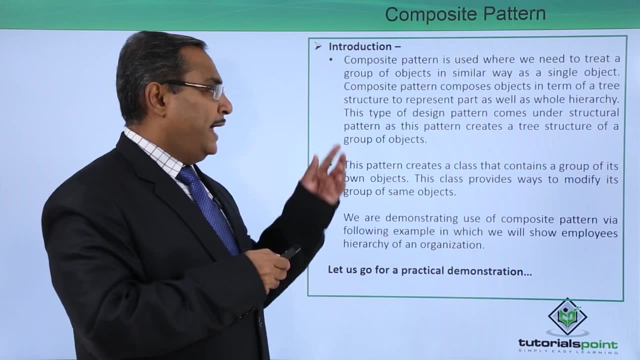 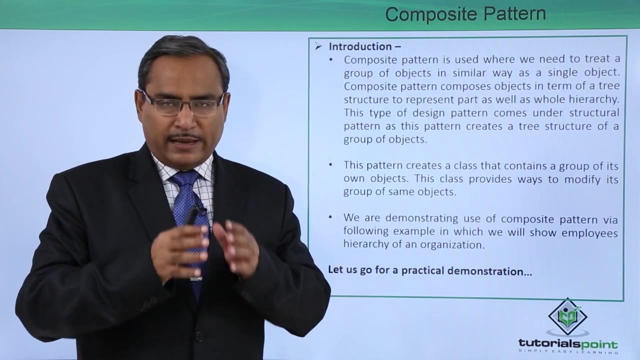 tree structure to represent part as well as whole hierarchy. This type of design pattern comes under the structural design pattern category, as the pattern creates a tree structure of a group of objects. So that is the basic theme which is lying behind this design pattern, This pattern. 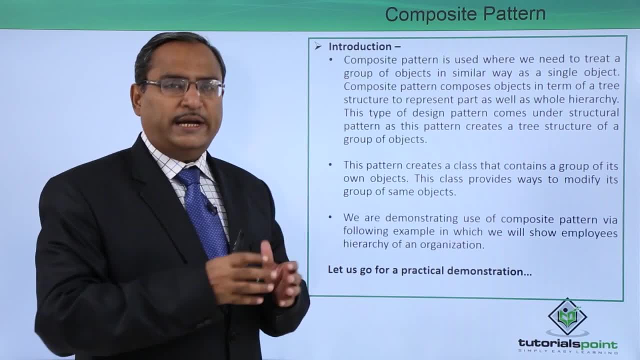 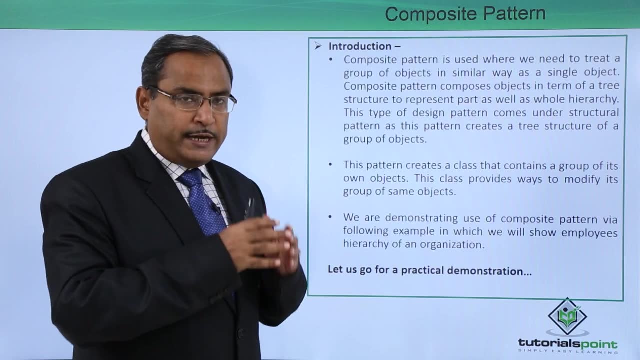 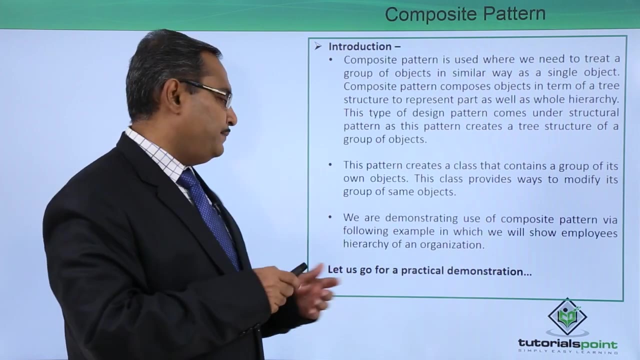 creates a class that contains a group of its own objects, and this class provides ways to modify its group of same objects. So we shall be creating one class and this class will be containing a group of its own objects. inside The class definition, We are demonstrating use of composite pattern via following example: 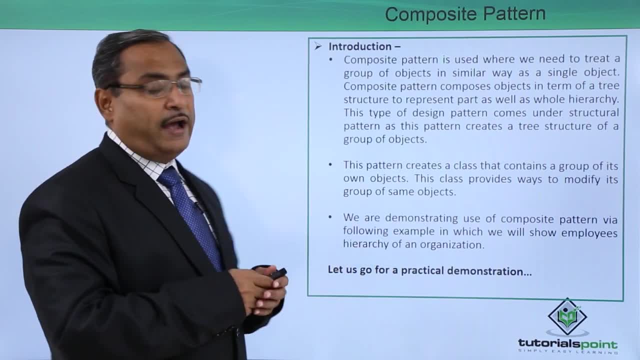 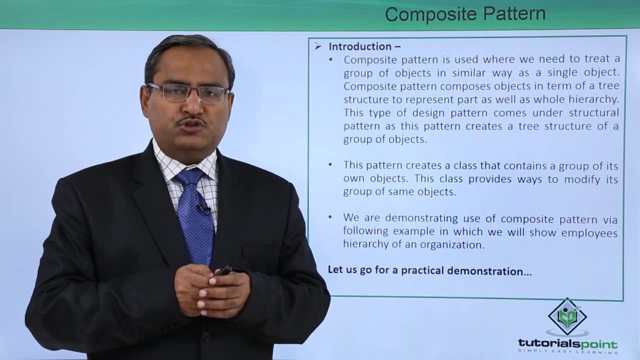 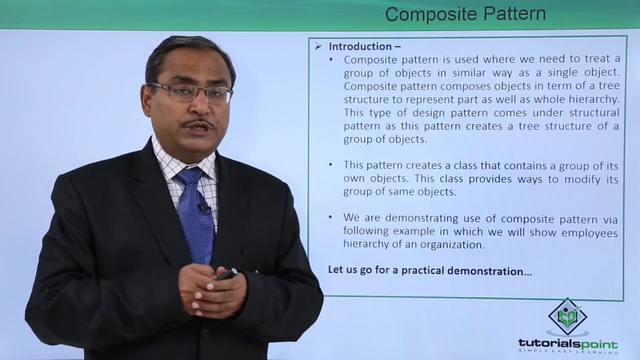 in which we will show employees hierarchy of an organization. So there we will be, finding one tree structure. So let us go for one practical demonstration, using Java programming language to develop one application on this composite design pattern demonstration. So here is the demonstration for you. 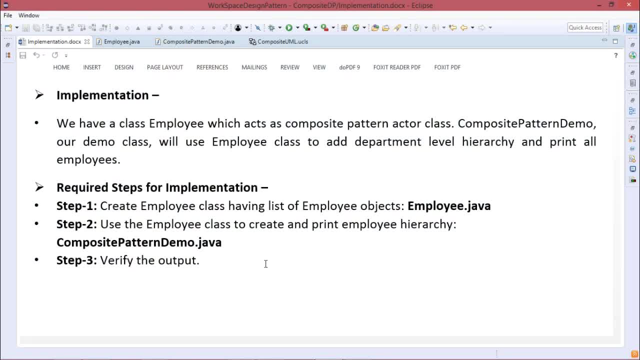 In this implementation. we are going to show you some Java code to implement composite design pattern. So we will be having one class- The name of the class will be employee, which acts as composite pattern actor class, and composite pattern demo will be our demo class, which will use this employee class to add department level hierarchy. 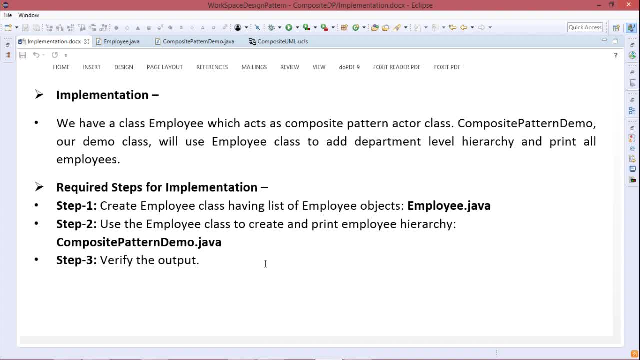 That means one employee under another employee under another employee. In this way there are some hierarchical structure depending upon the designations and print all the employees accordingly. So let us go through some steps. So step 1,, step 2 and step 3.. 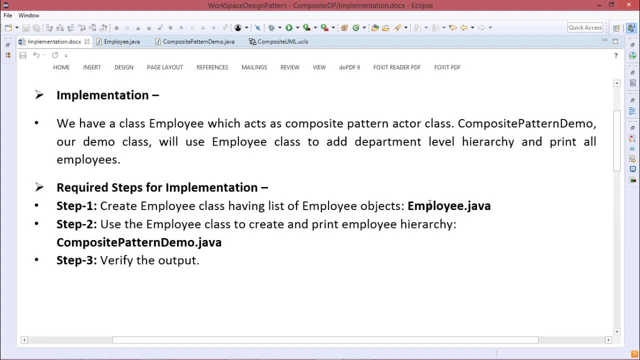 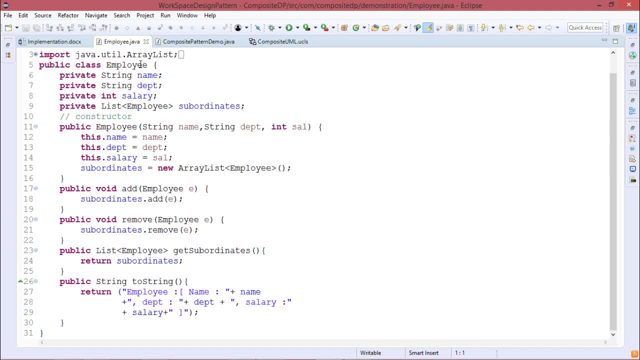 Step 1. Create employee class having list of employee objects in employeejava. So let us go for step 1 at first. So here we are having one class. The name of the class is employee, Having got instance variables, that is the name of the type string department, of the type string salary, of the type integer. 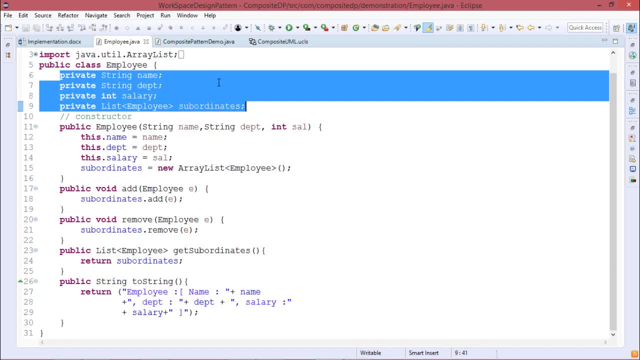 We are having one subordinates of the type add a list, So this particular subordinates can hold employee class objects. so employee is nothing but one constructor defined under this class, employee which takes this name, department and cell as input arguments to initialize this instance. 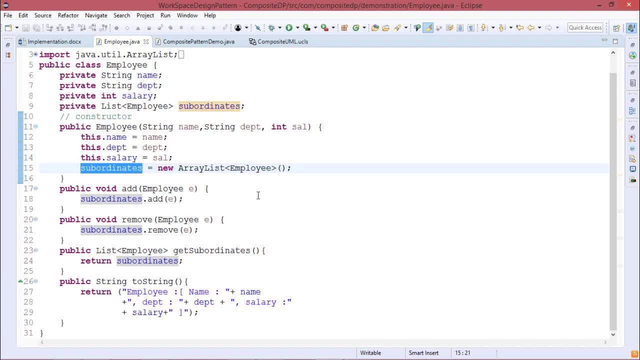 variables. we're having this subordinate. so what is the subordinate? that is a. there is a add a list object, so is equal to new add a list which can contain the employee class objects as in as add as its member. so now we are also having this add method. so add employee e. so subordinates dot add e. 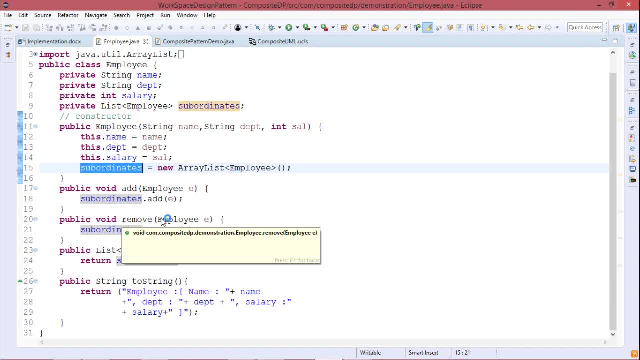 we are having this remove method, that is, a remove the employee e, which removes this employee e from this subordinates at a list. so also we are having the get subordinates and is another method which returns the least employee and there is a return subordinate. so subordinates will be returned. 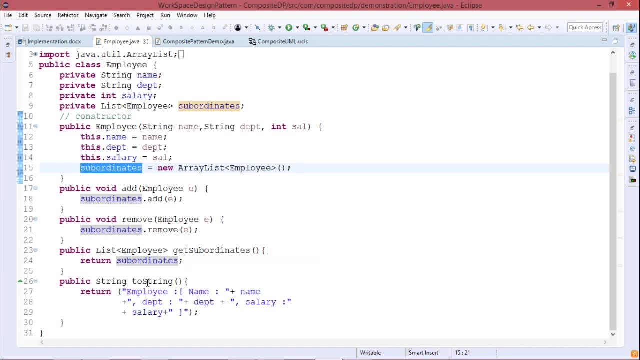 from this get subordinates method. we're having the method that is a two string and this method is actually printing the name, the department, the salary as well. so for this we are writing this two string method. so again, I'm repeating: so we are having one class, the name of the class is employee. having got this instance, 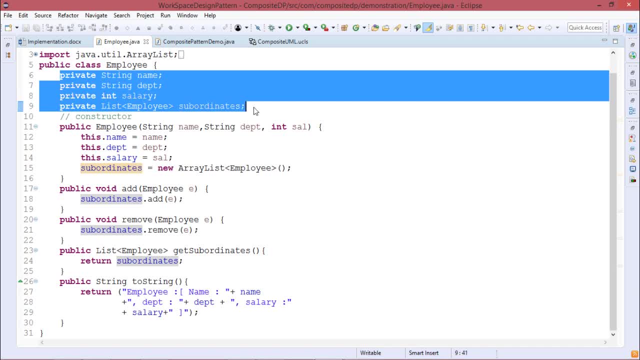 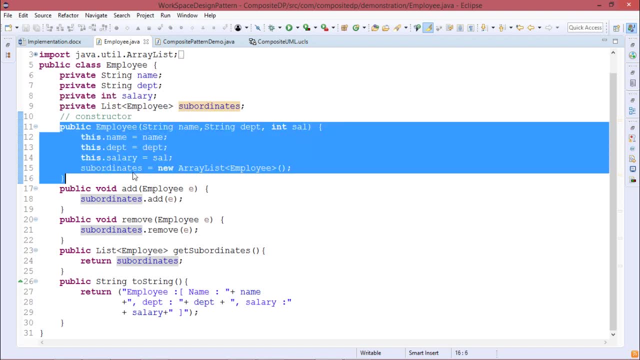 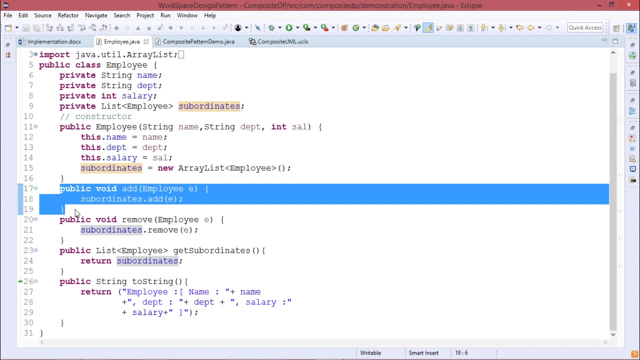 variable. also, we are having another instance variable. there is a subordinates, which is of the type: add a list which can hold employee class objects. so this is the constructor to initialize all the instance variables, all the four instance variables. so this is the add, which will add a new employee object to the 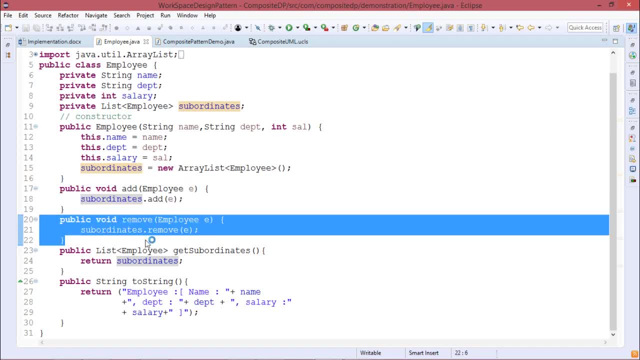 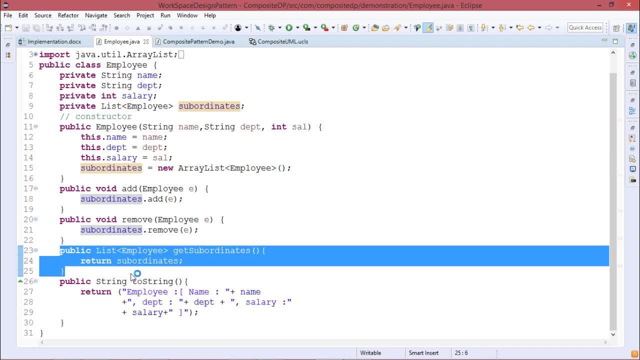 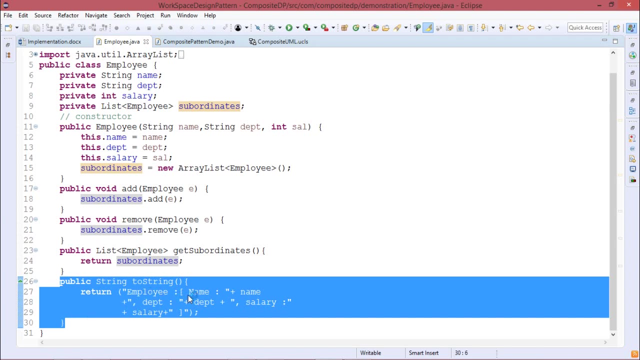 subordinates at a list. this is a remove which will remove the employee object from the subordinates at a list. so this is the get. subordinates is a method which returns the add a list. there is a subordinates and there is a two string method which will print the name, department and the 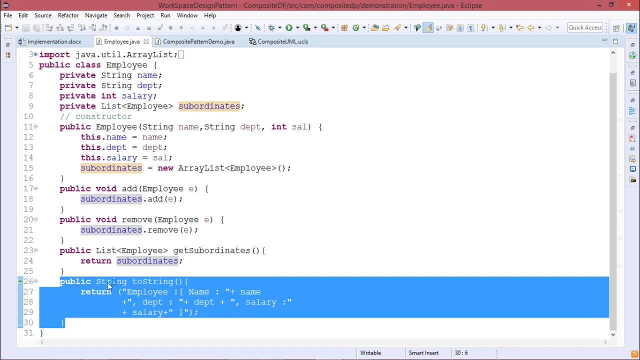 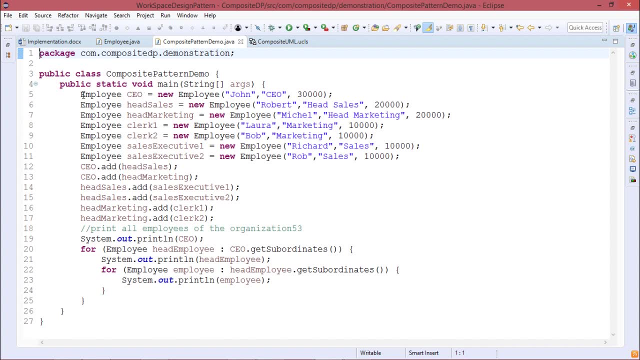 salary in a certain string. so it's a string will be returned and that can be printed later on. so now we are having this composite pattern, demo dot, java. so we are defining one employee object, that is, a ceo. we are having these head cells: head marketing clerk, one clock, two sales executive. 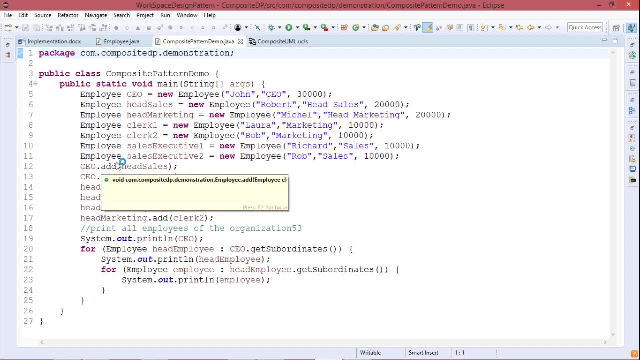 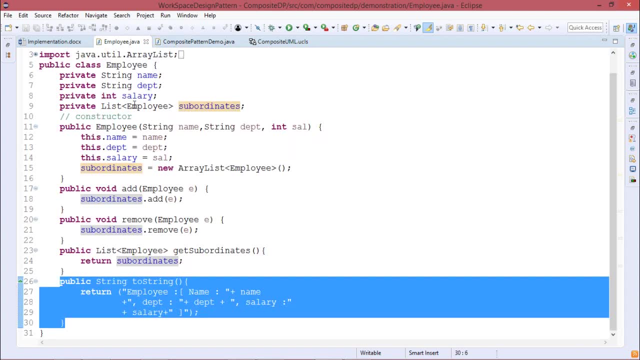 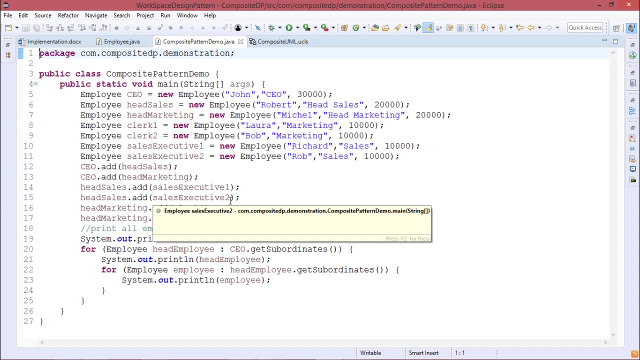 one, and sales executive two. so each one of them are of the type employee, so the all of them are employee class objects. so all of them are having their own and there is a analyst that is the subordinates. remember this one. so now we are going for this hierarchical- uh organization that is the. 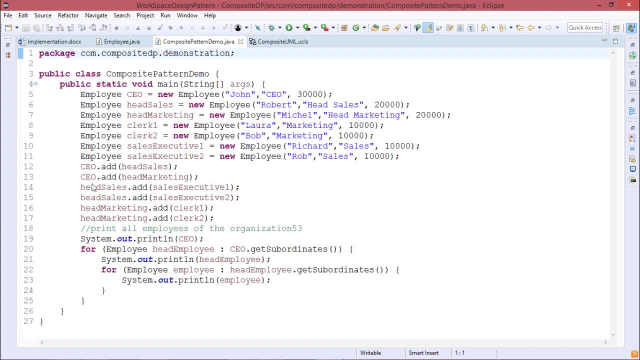 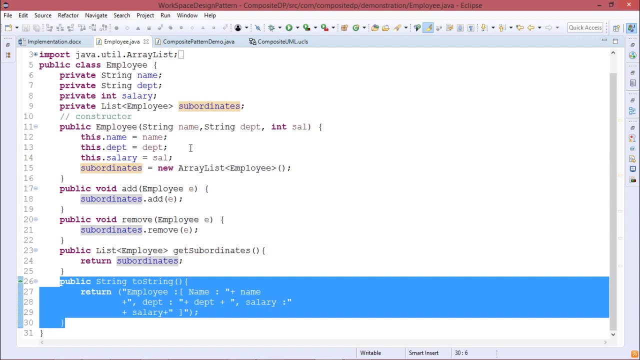 and that is a who will be working under whom. so ceo dot ad head cells. so this employee, this employee object head cells will be, will be there in the add a list of this ceo. so ceo is of the type employee, employee, class, object. so the add a list is known as a subordinate. so that's why. 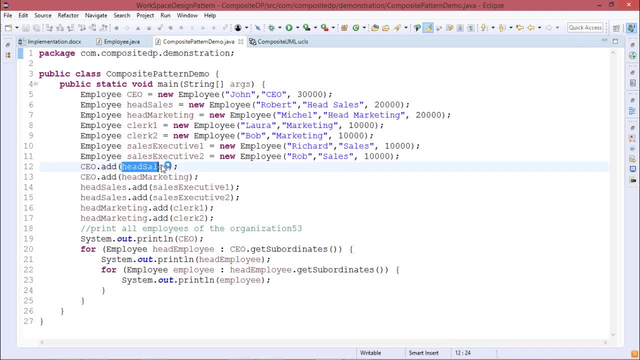 this particular ad will will include these head cells in the subordinates, add a list and define under the uh, under the object ceo, employee, object ceo. so ceo. dot add head marketing. then head cells: dot. add sales executive: one head cells dot. add sales executive. two head marketing dot. add clerk: one head marketing dot. 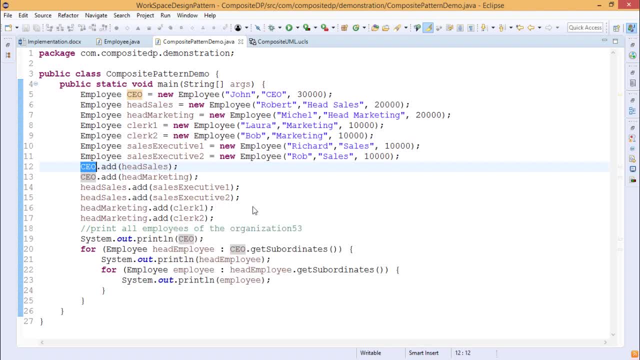 add clerk two. so you are getting one designation hierarchy here. and there is a main feature of this composite design pattern. so now we are printing, printing this ceo, so we are just printing this one. so when you are printing one object, then object name dot to string method will be executed. 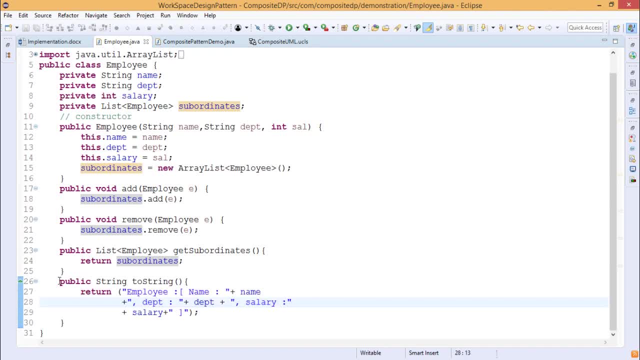 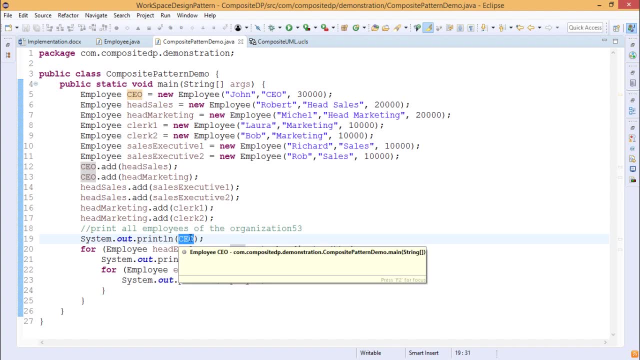 so as a result of that method, which is having the prototype, that is, a public string, true string, This particular method will be executed. So co will print: will get the object content: co. employee object content: will be printed accordingly the respective member variables. 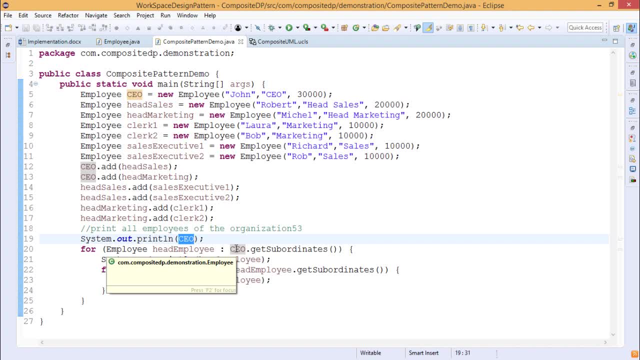 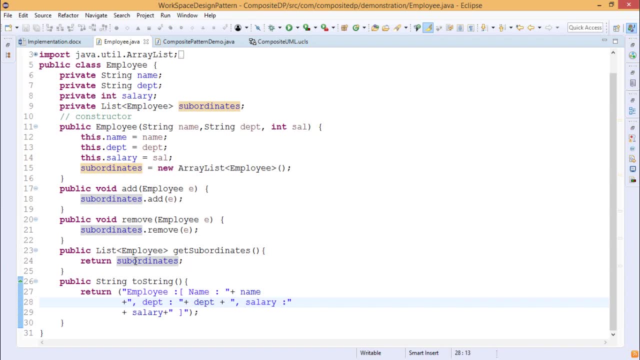 So now we are having this employee head employee colon- this is my co dot- get subordinates. you know that in case of get subordinates, it is returning the full subordinates. that is the. that is the add list. it will return this add list subordinates. 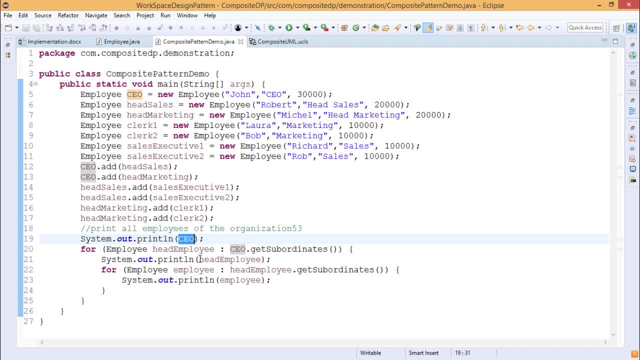 So from there it will go on printing the head employee details. So what will happen? if you are, when you are printing this employee object, head employee, then head employee dot. true string method will be executed And for each and every head employee we are going to print its subordinates. 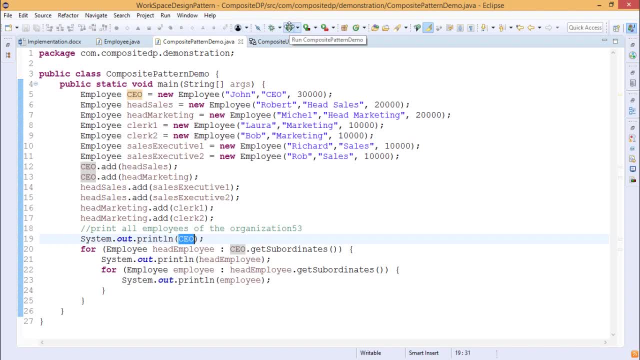 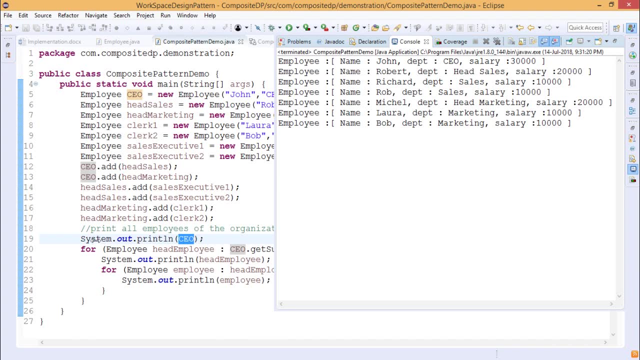 So in this way we are going to print here. So now let me go for the execution. So, employee name: so this is the john department co salary, this, so this line is getting printed from here. And then we are having this one that is a head sales. 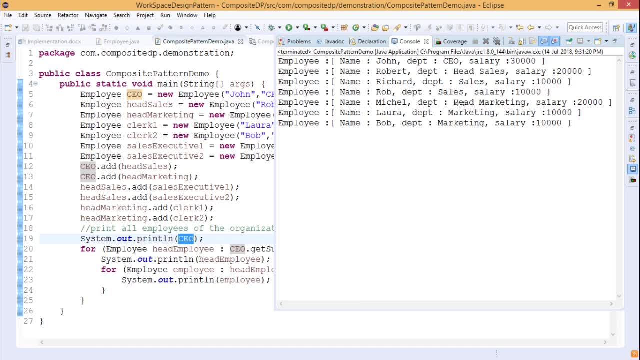 So under these head sales- so we are having this- two persons are working in the sales department, then head marketing and two persons are working in the marketing department. So they were defined as a clerk one and clerk two. So here you can find that they are working under the marketing department. 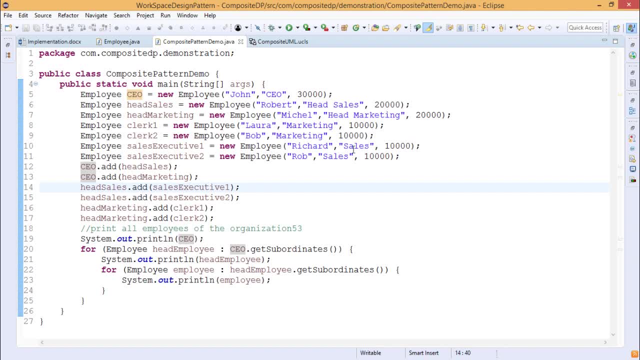 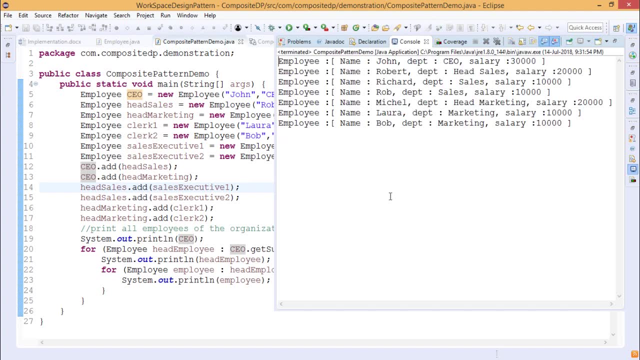 And this is my head marketing here. We are having this one. they'll be working in the sales department. So, accordingly, the outputs are coming, So this output. you can easily find that, how these outputs are coming. outputs are coming and these outputs are coming, depicting that this add, how this add took. 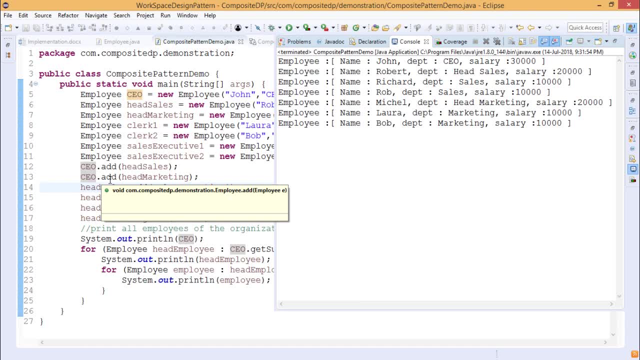 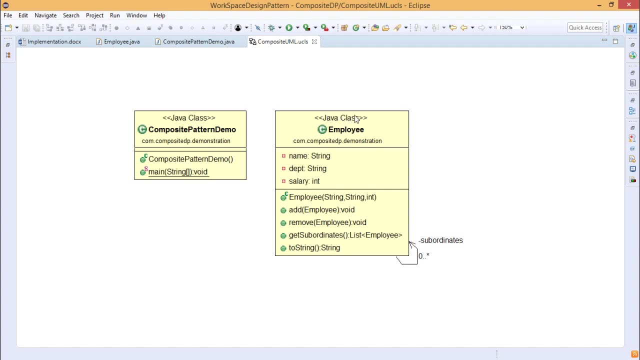 place to have that designation hierarchy getting formed in the memory. So I think now the concept is clear to us regarding this composite design pattern. So now let us go for the class diagram here. So here we are having this employee, that is a Java class we are having and it is having 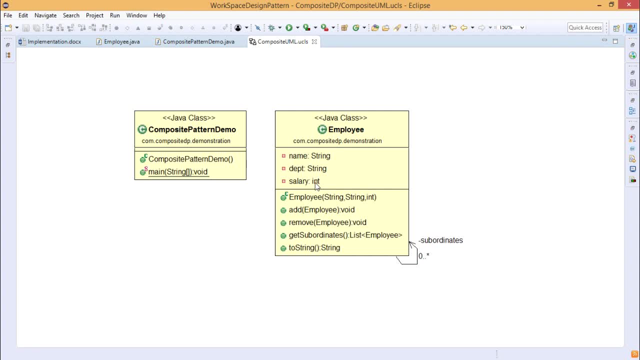 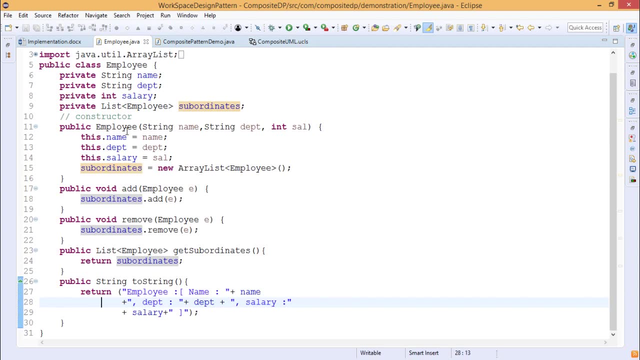 the respective member variables, that is, the name, department and the salary, and this is one having one subordinates we are having, So these are our employee, so subordinates are there and it is under the private scope and that is why we are having this minus symbol there. 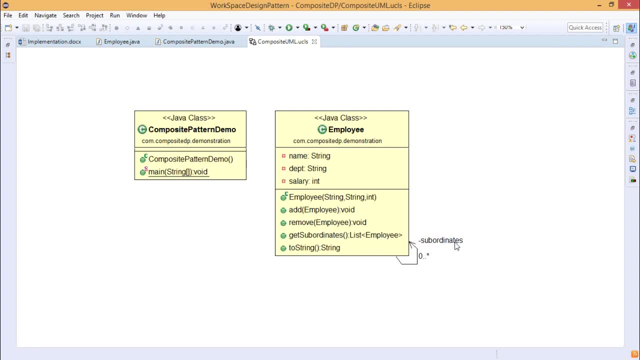 The subordinates is of the type Adelies can contain multiple employee objects, So zero to many employee objects can be kept in the subordinates, But having this employee constructor defined under the public scope. We are having this: add method, remove method, get subordinates method and true string method. 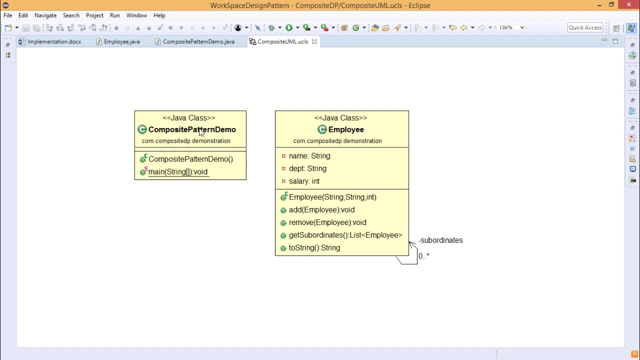 all of them are under the public scope. We are having this composite pattern demo class and which is having the composite pattern demo constructor and the main method, which is public static. So in this way, in this particular video, we have discussed how this composite design pattern.